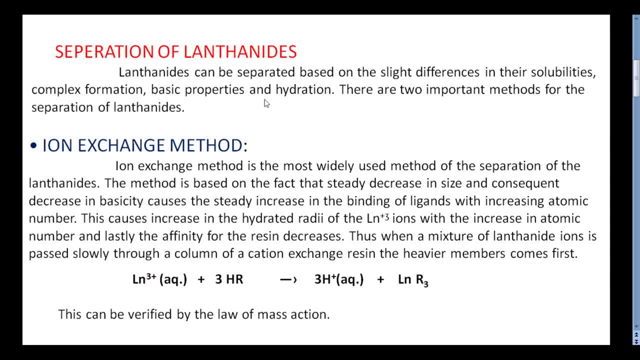 solubilities, complex formation, basic properties and hydration. There are two important methods for the separation of lanthanides. Lanthanides can be separated based on the slight differences in their solubilities, complex formation, basic properties and hydration. 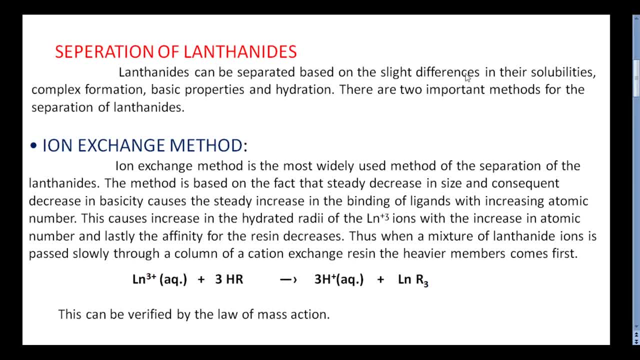 So, based on these four properties, we can separate lanthanides based on the slight differences in their solubilities. So to separate lanthanides there are a number of methods. There are two important methods. First one is ionic separation. 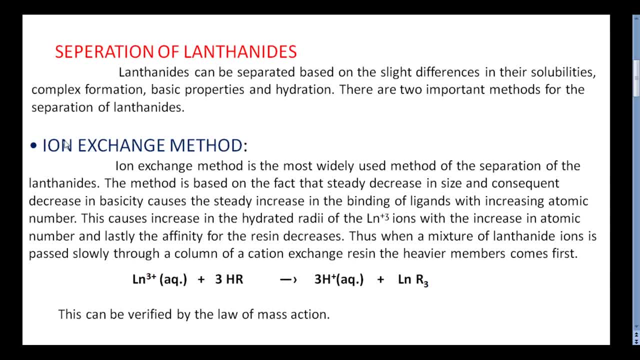 Second one is solvent extraction method. So first the ionic separation method. Ionic separation method is the most widely used method of the separation of the lanthanides. The method is based on the fact that steady decrease in size and consequent decrease in 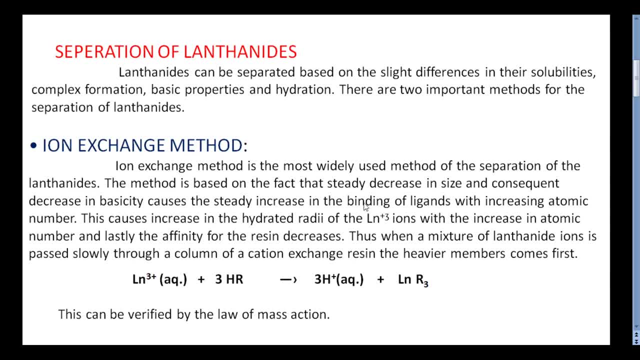 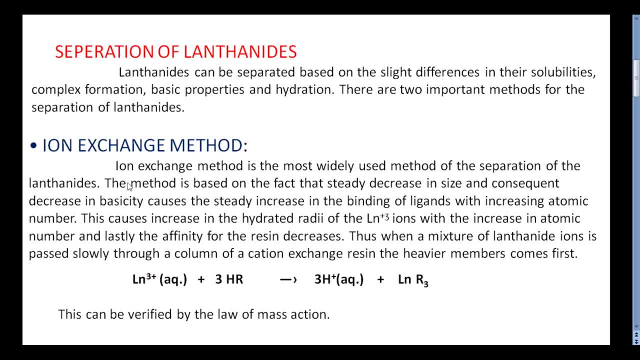 used for separation of lanthanides. So this method is based on study. decrease in size and consequent decrease in basicity causes the steady increase in the binding of ligands with increasing atomic number. So already we have said in lanthanide contraction that if atomic number 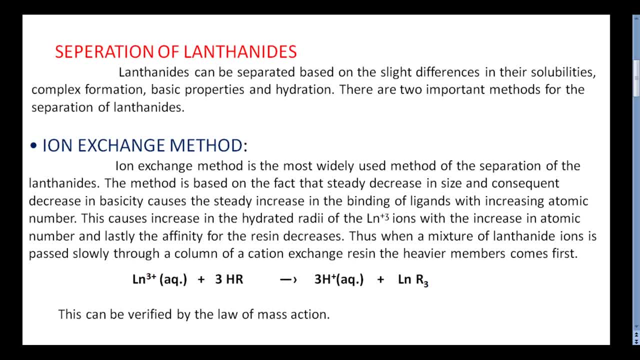